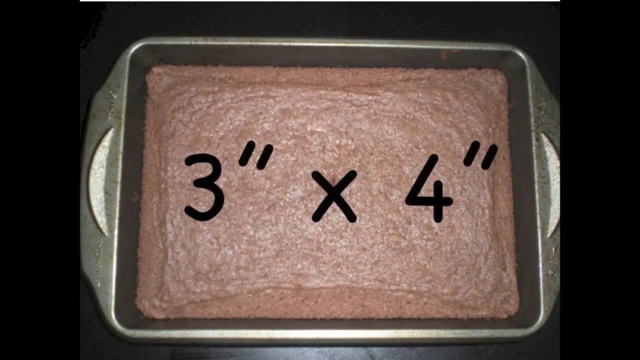 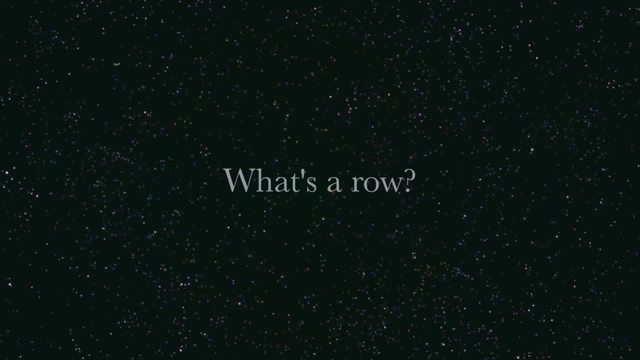 Remember when we said that the pan was 3 inches by 4 inches. Well, let's try this. Why don't we divide the pan of brownies into equal-sized square pieces using rows and columns? What's a row? A row is when parts of a shape go across. 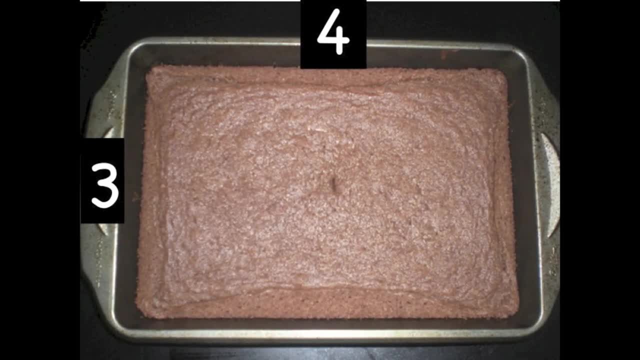 Here, let me show you. Let's try breaking this brownie pan into three rows, or three pieces that go across One row, two rows and three rows. This can sometimes get confusing, because we only made two long slices, But now there are three long parts. 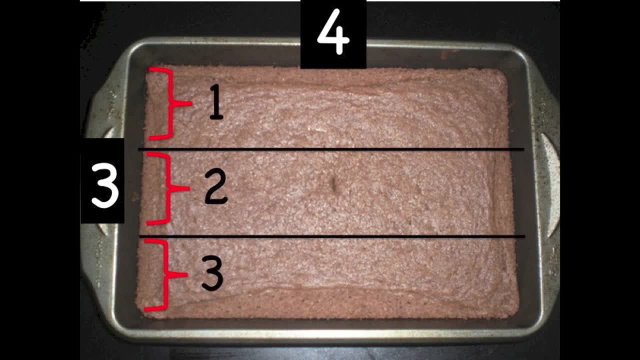 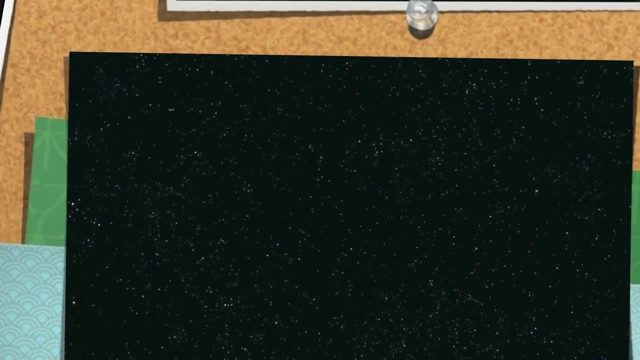 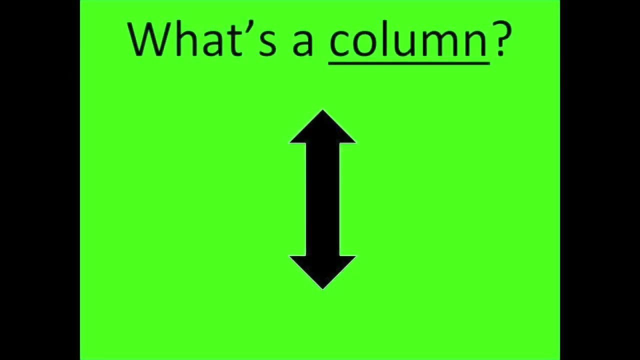 Three parts that go across, And remember we call these rows. Now let's divide our brownie into columns. What's a column? Columns are parts of a shape that go up and down. Let's divide our brownie into columns. 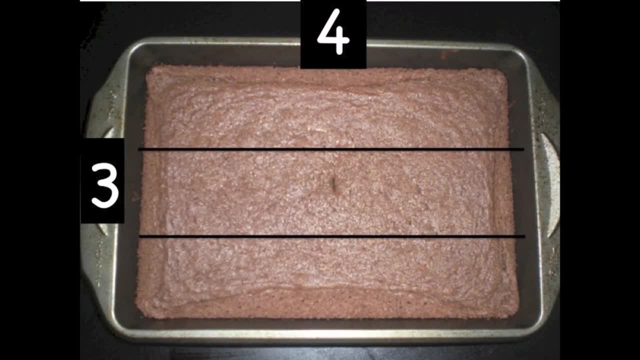 I'm going to put columns on top of the rows that I've already cut into my brownie. I will divide my columns with the color white. We've got one column, two columns, three columns and four columns. Remember, this is the part where it can get a little tricky. 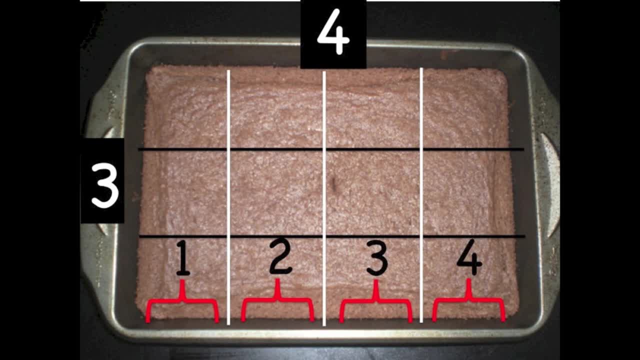 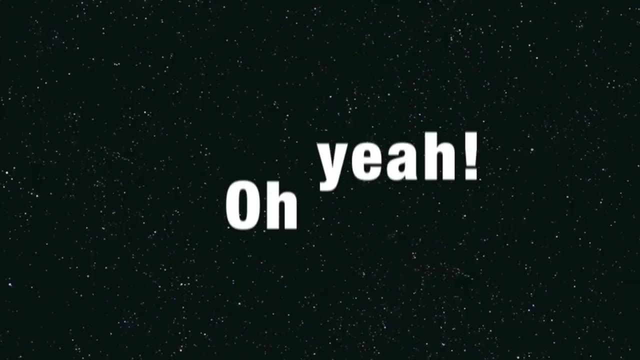 We made only three cuts with the white line, But we have one, two, three, four columns. So remember, we were trying to break our pan of brownies into smaller and equal sized squares. Well, did we do it? Oh yeah, 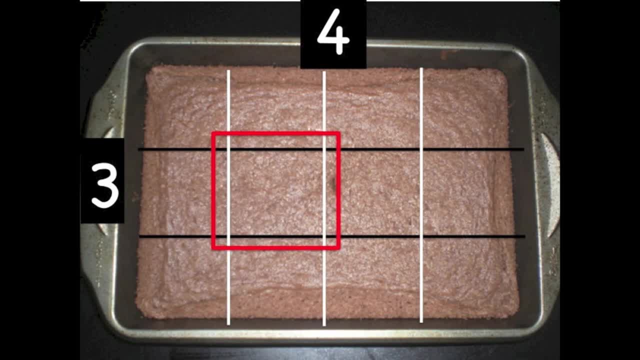 I think that this shape looks like a square And it looks like it's the same size as this other square- Great job. I think that all of these pieces look like squares And they all look like they're the exact same size- Great. 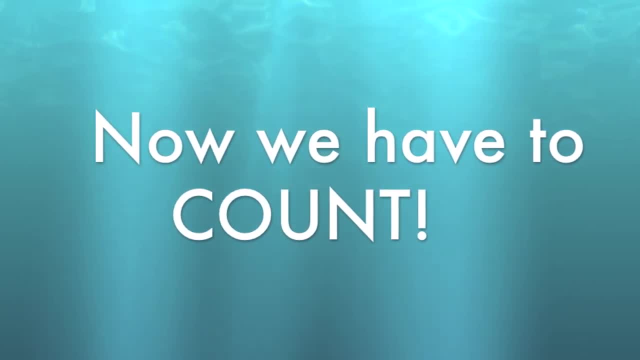 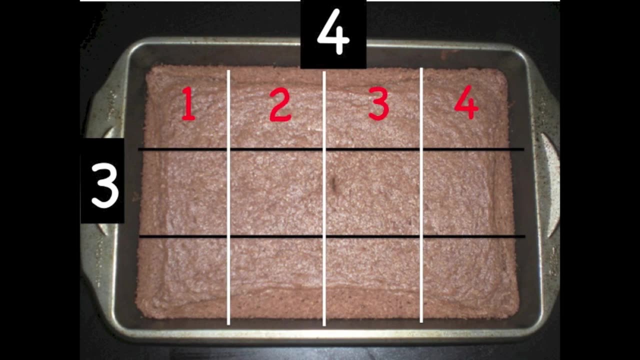 Now we have to count. How many pieces of brownie do we have now? Let's count together: One, two, three, four, five, six, seven, eight, nine, ten, eleven, twelve. We divided our brownie into twelve equal, same sized squares.